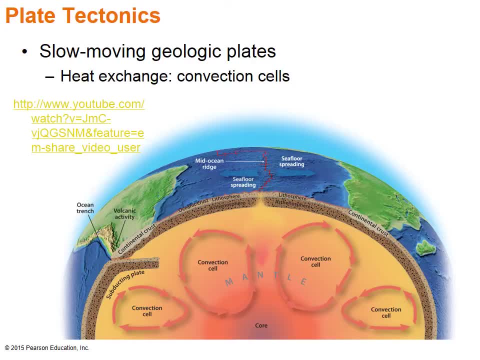 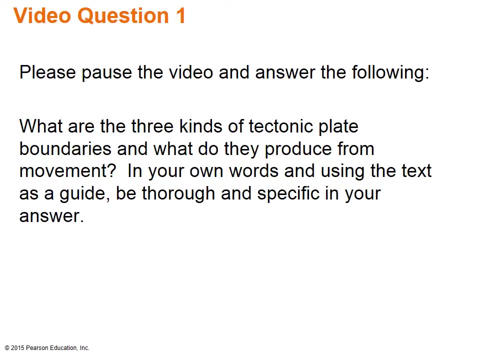 by plate movement along the boundaries. Please pause the video and click on the link to watch a video on plate tectonics. Be sure to take notes in order to help you answer the question on the next slide. What are three kinds of tectonic plate boundaries and what do they produce from movement? 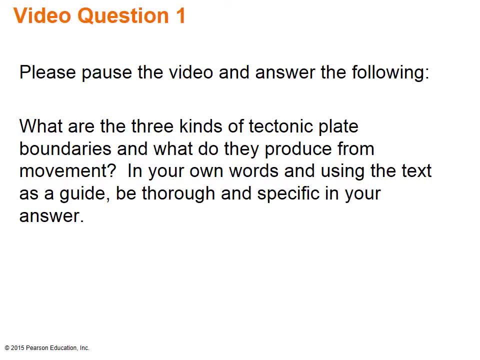 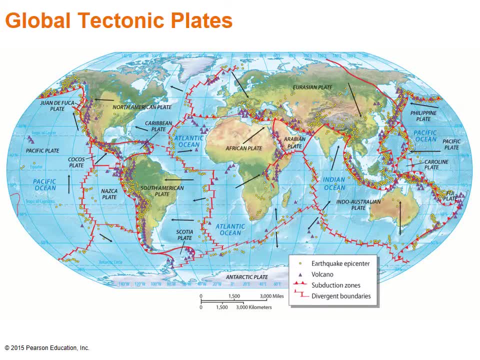 This map of the world shows the close relationship between tectonic plate boundaries and the world distribution of earthquakes and volcanoes. Think of the Earth as a place of movement. This is just a single example. You might use it as an example, but it is not clear enough. Please pause the video and answer the following: What are three kinds of tectonic plate boundaries and what do they produce from movement? Provide an example for each In your own words and using the text and video as a guide. be thorough and specific in your answer. 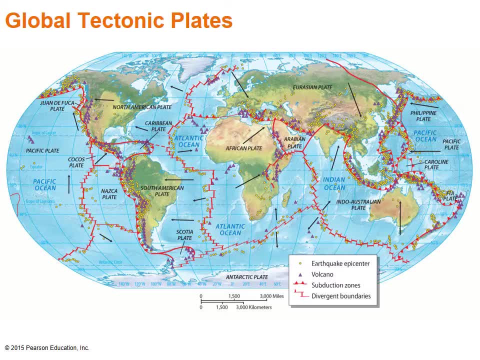 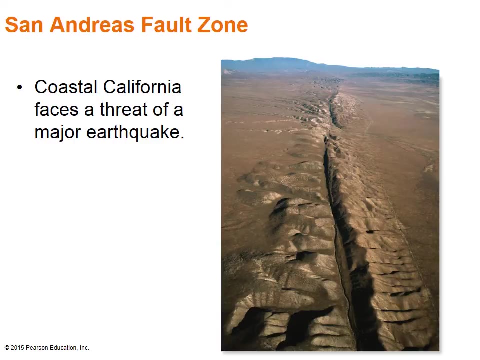 Note the so-called Pacific Rim of Fire that includes the eastern coasts of Asia and the western coasts of both North and South America. The San Andreas Fault has long been thought of as a place of convergence of the North American and Pacific plates and was originally formed by two plates colliding. 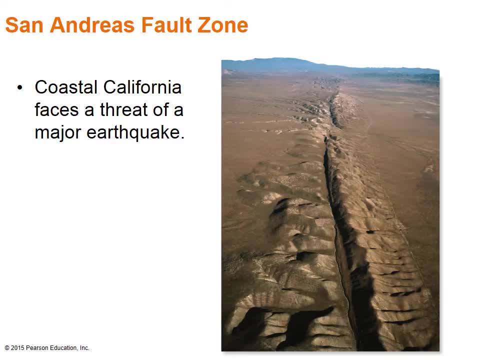 However, in recent years, some geologists believe that this place of convergence is really to the east of the Sierra Nevada mountains. More recently, this fault became a transform fault, where the eastern edge of the Pacific Plate moves laterally northward at a rate of several inches per year, pushing sideways. 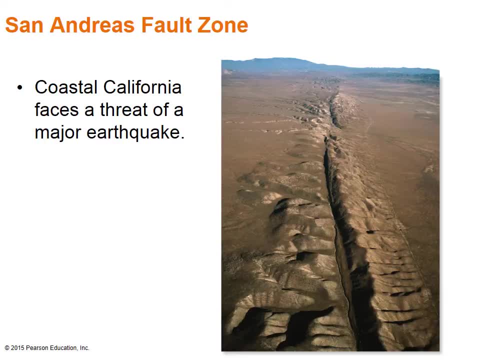 against the North American Plate. The photo is of the main fault trace of the San Andreas and Dry Carrizo Plain area, halfway between San Andreas and Pacific Plate. The San Andreas and Dry Carrizo Plain area is located in San Francisco and Los Angeles in the California Coast Ranges. 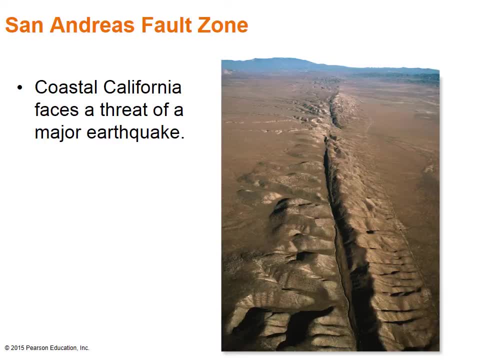 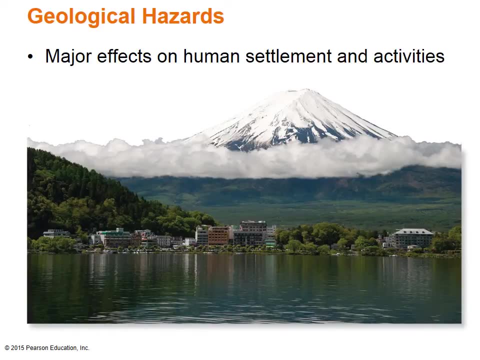 This area has always been a hotspot of earthquake activity, and especially for the two cities. There are several major geological hazards that have had an effect on human activities. They include earthquakes and volcanoes, and occur primarily along the plate boundaries. The photo shows Mount Fuji, the highest mountain in Japan, at almost 13,000 feet. 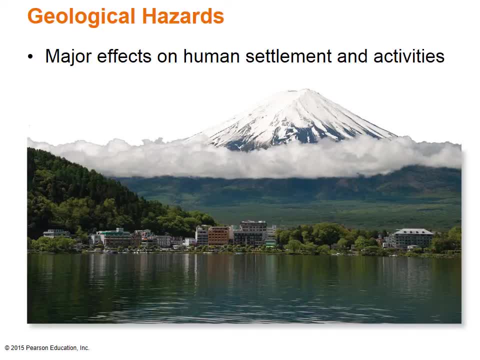 The photo shows Mount Fuji, the highest mountain in Japan, at almost 13,000 feet. The photo shows Mount Fuji, the highest mountain in Japan, at almost 13,000 feet. This is considered an active volcano and even though its last eruption was in 1708,. 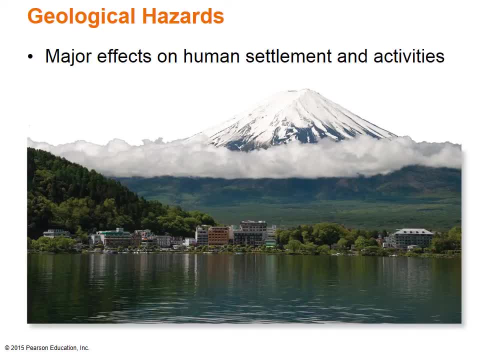 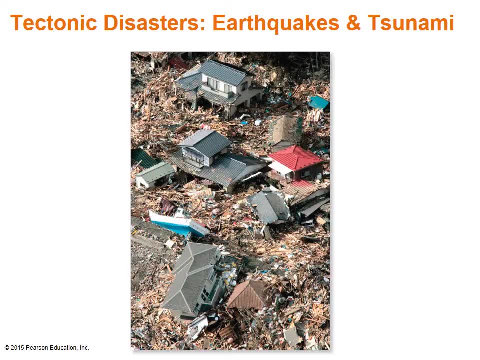 if this should erupt again, it would severely impact the 36 million inhabitants of Tokyo. just 60 miles away, The photo shows Mount Fuji, the highest mountain in Japan, at almost 13,000 feet. Tsunamis occur when massive earthquakes happen undersea. 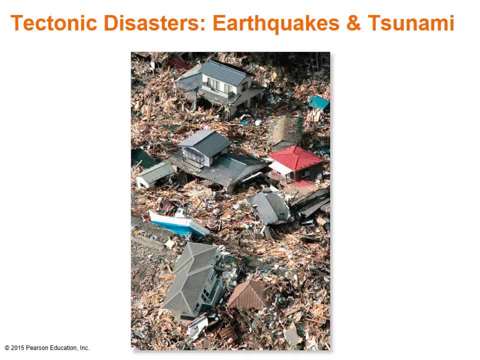 During an undersea earthquake, the energy produced from the earthquake is pushed up, creating a major ripple in the ocean and therefore sending huge waves towards the shore. During an undersea earthquake, the energy produced from the earthquake is pushed up, creating a major ripple in the ocean and therefore sending huge waves toward the shore. 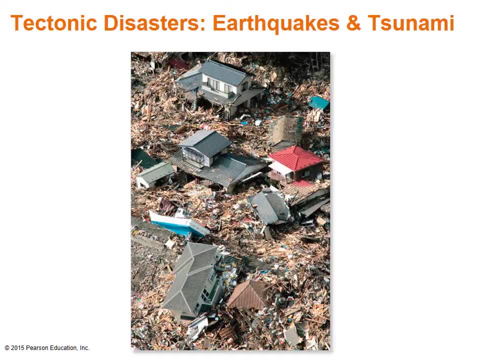 This is considered a very active volcano and, even though its last eruption was in 1708,, This photo shows the epic destruction of property along the northeastern coast of Japan that occurred in 2011,, when a major 9-point magnitude undersea earthquake generated a tsunami that 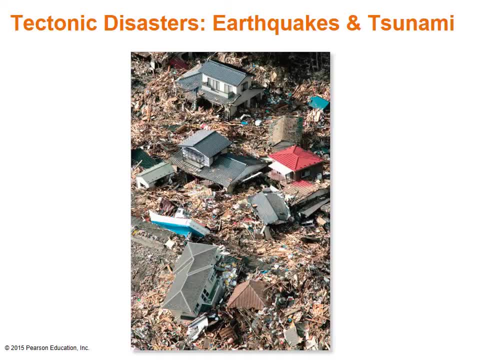 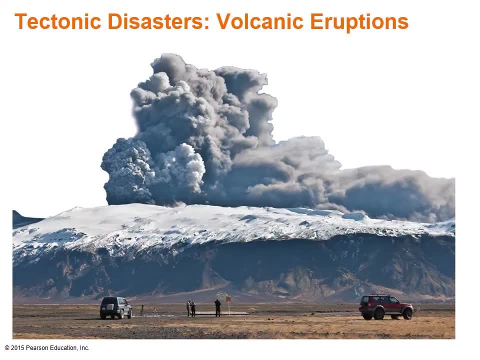 reached 133 feet high and traveled 6 miles inland, causing about 20,000 deaths. This photo shows the volcanic activity common in Iceland. because of the divergent tectonic border that bisects the island and the North Atlantic Ocean, This eruption that occurred in 2010 was the most notable for the major disruption to both. 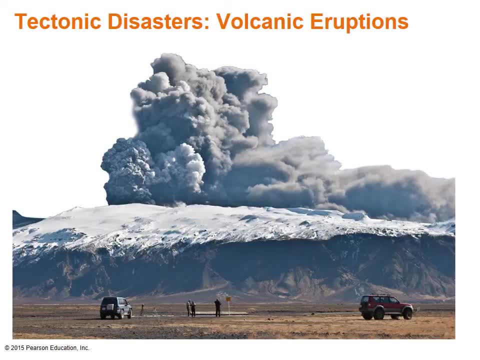 transatlantic and intra-Europe air traffic due to its ash carried by the wind. However, volcanoes can provide some benefit to people by producing geothermal energy to heat houses and power factories, and the ash can fertilize the soil for agricultural purposes. 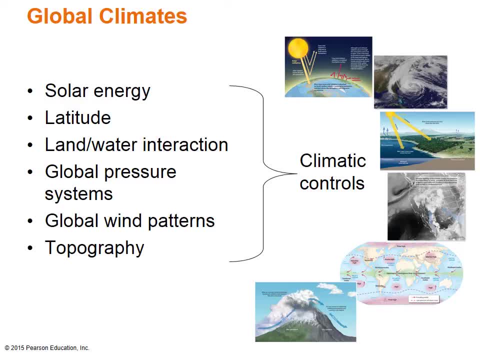 Most human activities are closely linked to weather and climate. Humans need the right temperature and moisture to grow crops, for foods and other products. Much of the world's landscape diversity results from ways in which people adapt to weather and climate. This adaptation will continue as climate and weather continues to change through processes. 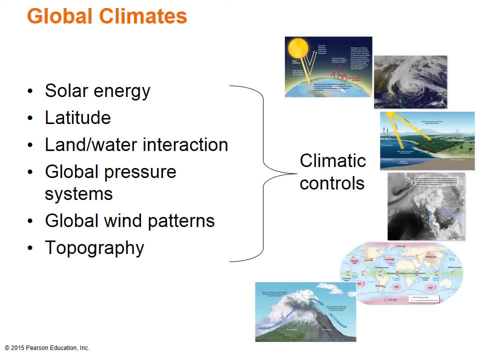 such as global warming. The world's climates differ from place to place as they are influenced by these climate controls, Solar energy, Latitude, Land Protection, Global pressure systems, Global wind patterns And topography. We will look at these factors in the next several slides. 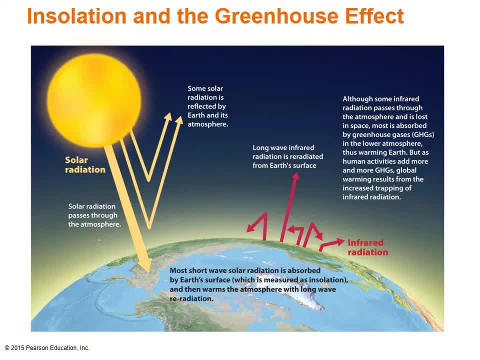 The natural warming of the Earth's surface is due to heat from the sun, called solar radiation. Solar radiation is the most important factor in the Earth's climate. Solar radiation also is responsible for driving other important processes, including global pressure systems, winds and ocean currents. 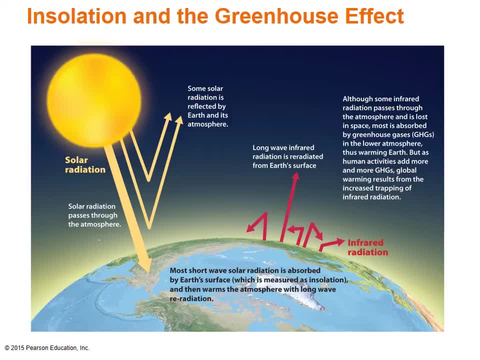 So how does all the heat from the sun stay near the Earth's surface? If it weren't for the greenhouse effect, solar radiation would bounce back off into space, causing much colder temperatures than we have now, much like that on Mars. Humans would not be able to live on Earth without the greenhouse effect. 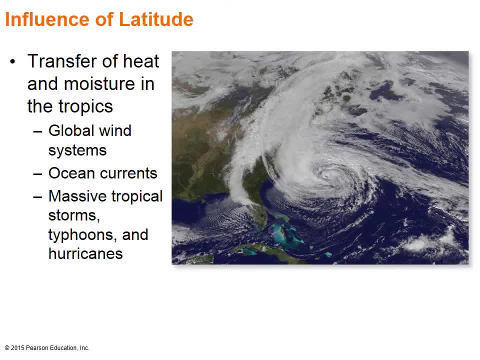 The influence of latitude also affects our climate and temperatures. In the past we have seen a lot of climate change, But how does all the heat from the sun stay near the Earth's surface? Insolation strikes Earth at different angles, which causes a differential heating of the 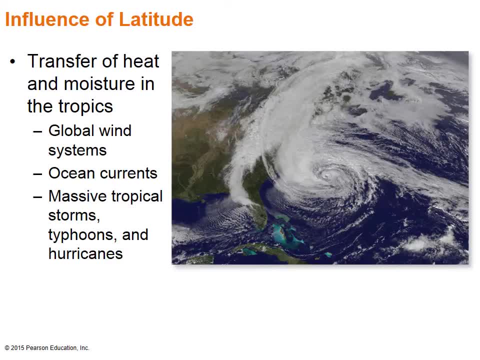 Earth's surface along the Earth's latitudinal lines. Latitudinal lines go north and south from the equator. In other words, solar radiation is more effective at or near the equator than from the higher latitudes toward the poles. Therefore, people experience solar heat more intensely if they were living near the equator. 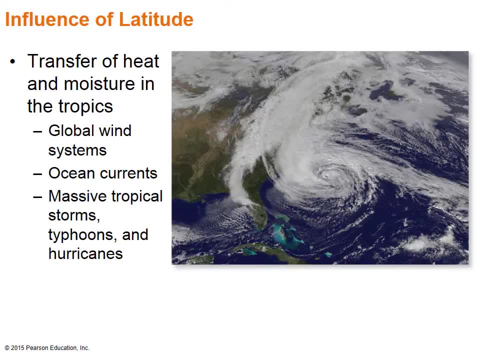 than people who are living closer to the poles. This heat is then redistributed away from the tropics through physical processes such as global pressure and wind systems, ocean currents, tropical typhoons, hurricanes and even mid-latitude storms. The photo shows Hurricane Sandy that devastated the east coast of the United States in 2012.. 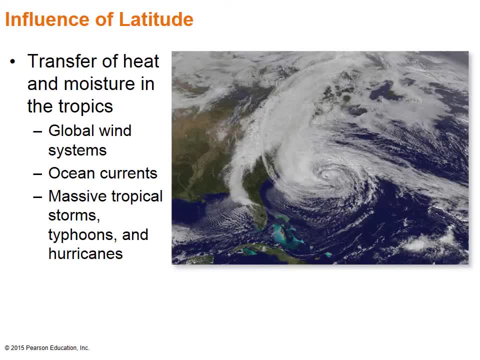 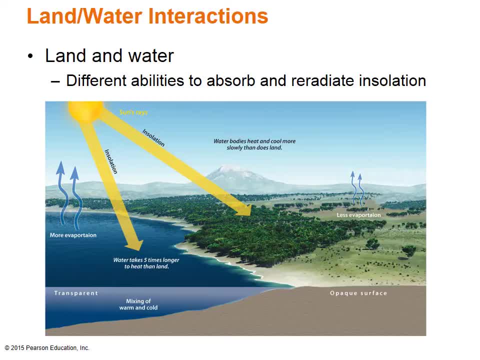 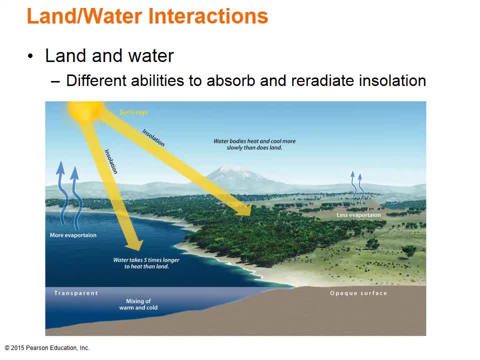 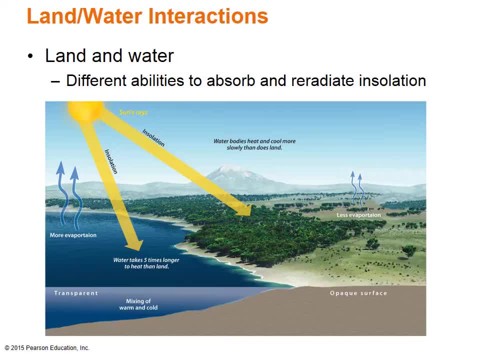 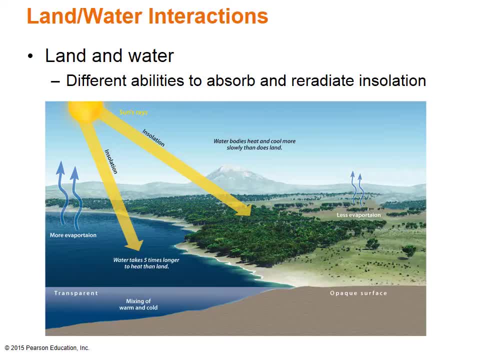 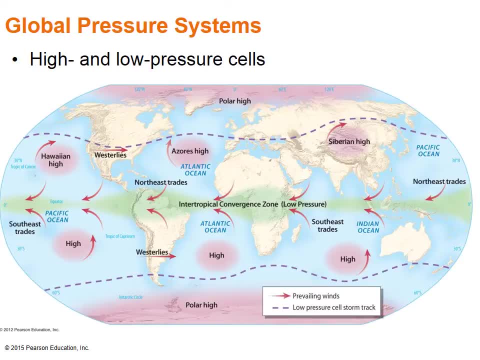 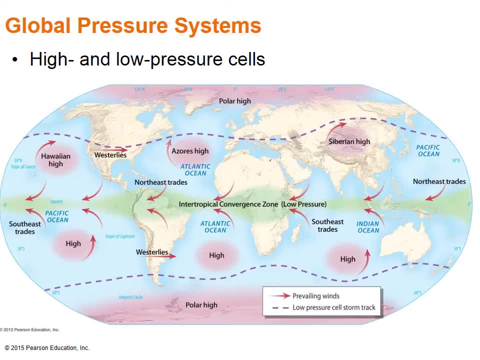 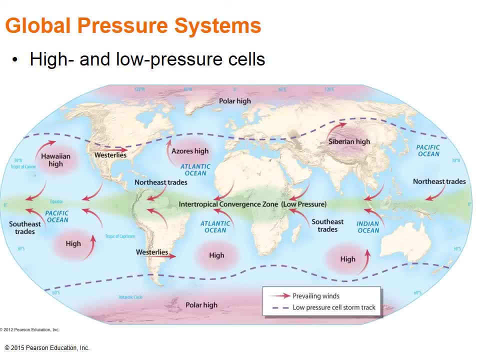 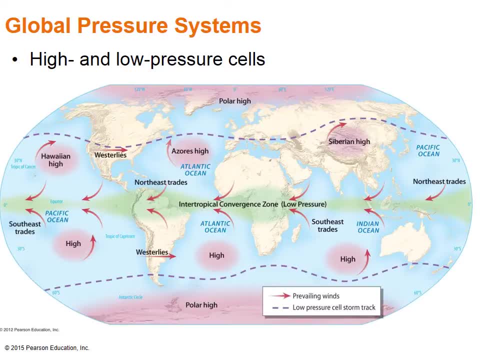 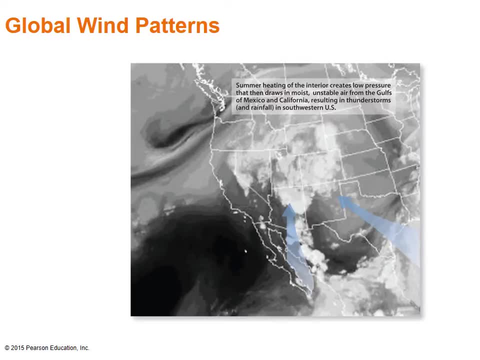 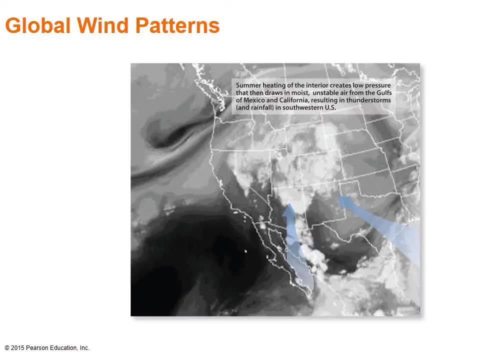 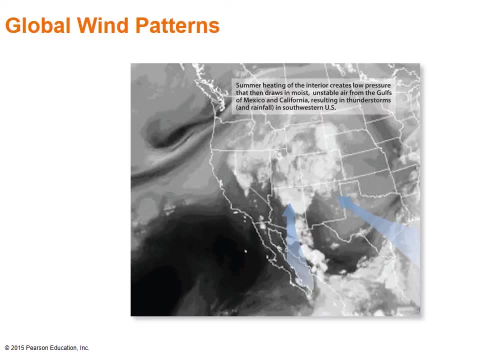 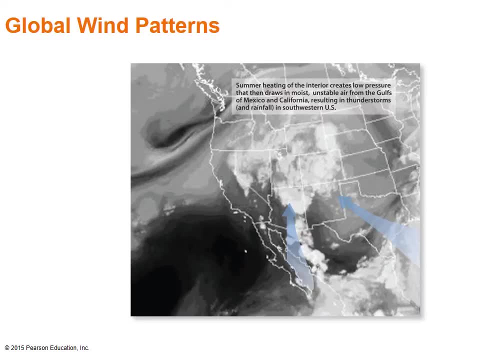 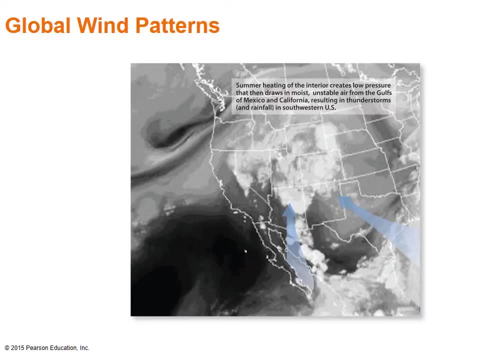 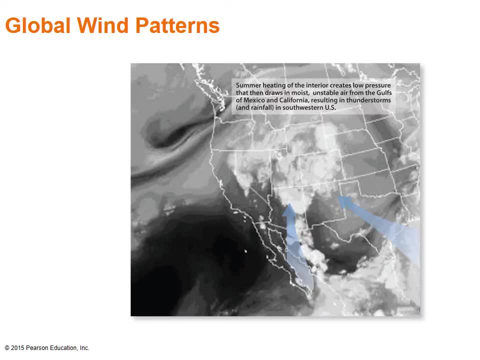 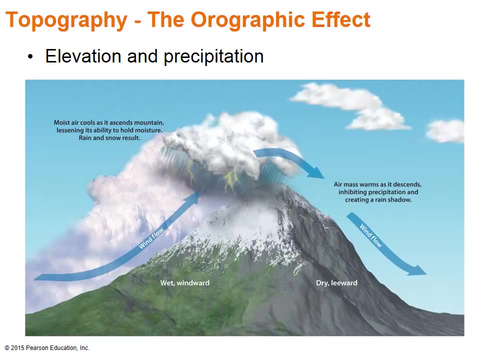 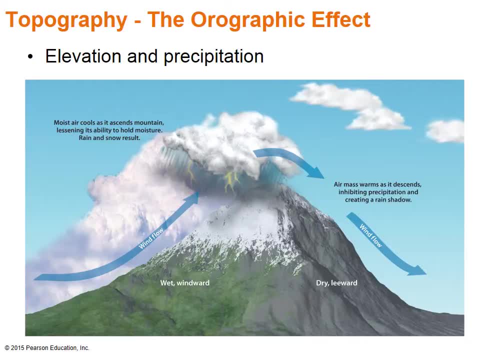 wet and dry areas. In this process, as air rises up the windward side of the mountain, it produces rain, fall and snow due to cooling temperatures at higher elevations where, as cold, air loses its ability to hold moisture, This cuts off what is in the slut of the family stream. 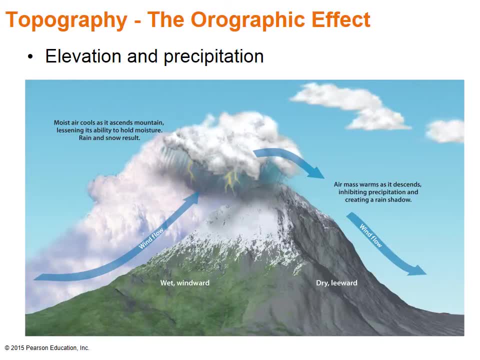 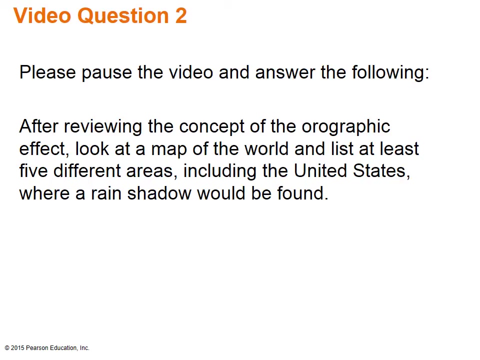 But once the air moves over the mountains, it begins to descend and warm up. Warm air has the ability to hold moisture, therefore leaving the leeward side dry. These dry areas are said to be in the rain shadow of the adjacent mountains. 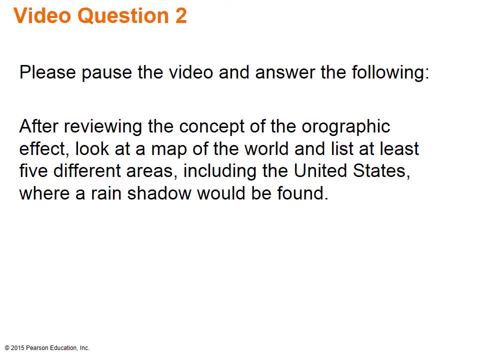 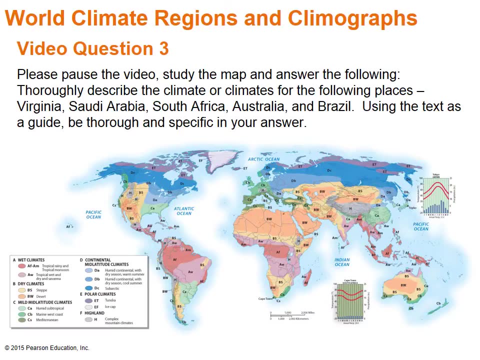 Please pause the video and answer the following. After reviewing the concept of the orographic effect, look at a map of the world and list at least five different areas, including the United States, where a rain shadow would be found. This map shows the world's climate regions in a few examples of a climograph. 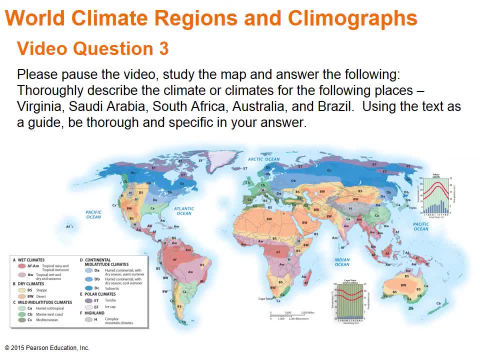 Climographs are graphic representations of monthly average high and low temperatures and monthly precipitation amounts. The climate mapping scheme that you see was devised to show the diversity of the world's climates. The difference between climate and weather is that climate and weather are different. Climate is a long-term average from daily weather measurements, while weather is the. 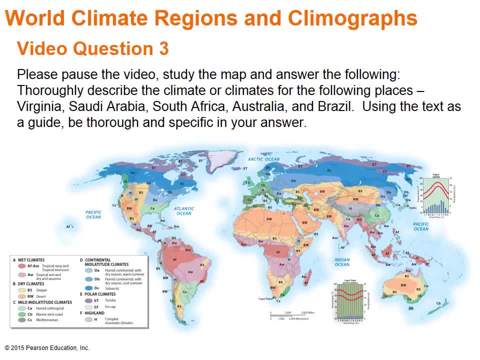 short-term day-to-day expressions of atmospheric processes, like: is it raining, cloudy, sunny, hot, windy or calm Weather, is usually measured hourly each day. In the map, a combination of upper and lower case letters describe the general climate. 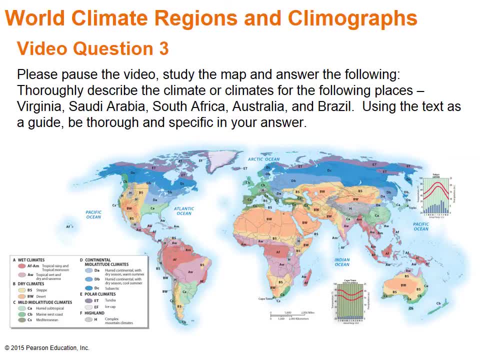 type, along with precipitation and temperature characteristics. Please pause the video, study the map and answer the following: What is the climate? What is the climate or climates for the following places: Virginia, Saudi Arabia, South Africa, Australia and Brazil? 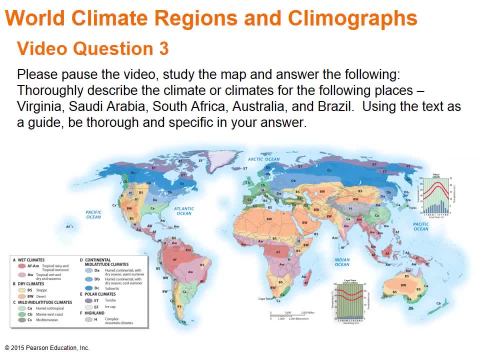 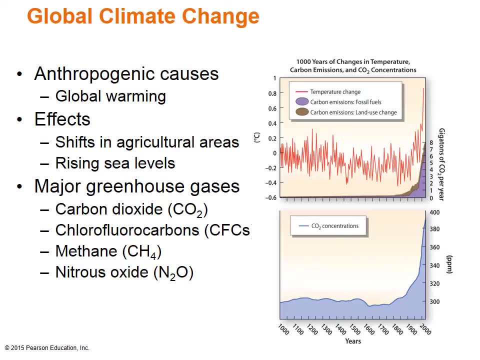 Using the text as a guide. be thorough and specific in your answer. The climate of the Earth has been warming naturally since the last ice age, but today the Earth's climate is warming up at alarming rates. Human-caused or anthropogenic activities are what is causing this change in ways that have 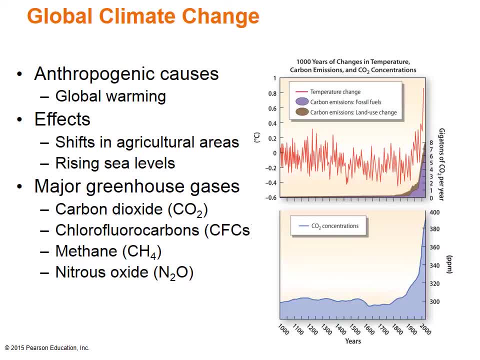 a significant impact on the environment. Specifically, pollution caused by burning of fossil fuels and the excessive emissions of the greenhouse gases listed are creating an imbalance in the greenhouse gas effect, which is in turn creating a warmer atmosphere than normal. This accelerated rate of warming, unlike the natural cycles of climate change itself, is 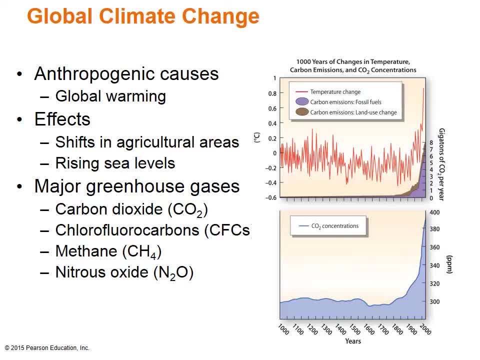 referred to as global warming. Global warming can lead to climate changes in such a way that it would change where and how we would produce food. It would also have effects on rising sea levels, therefore creating flooding in low-lying areas, just to name a few. 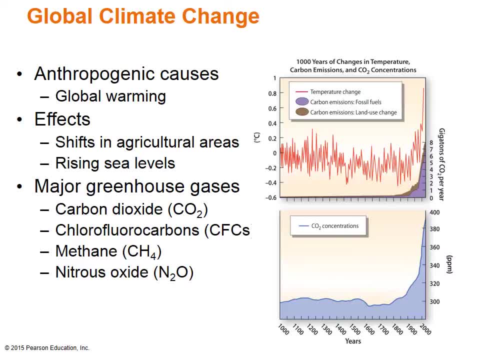 These two graphs show the relationship between the rapid increase in CO2 in the atmosphere and the associated rise in average annual temperatures for the world. Take a look at how far back these graphs go and examine how relatively stable the temperature and CO2 output have been until the recent industrial period began toward the 1900s. 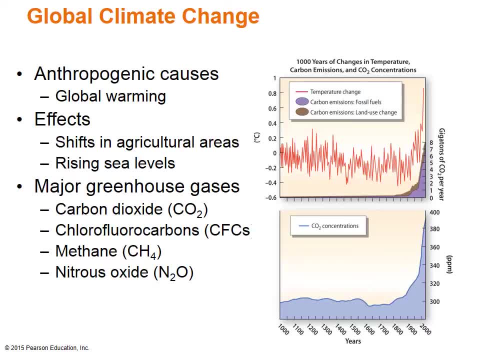 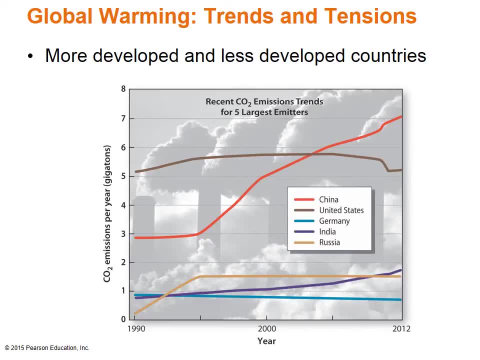 Thank you for watching. There are a few trends happening and tensions caused by those trends throughout the world regarding CO2 emissions and global warming. The graph shows that many of the fully industrialized, more developed countries have stabilized their CO2 emissions and, in some cases, have reduced them, whereas China and India have steadily. 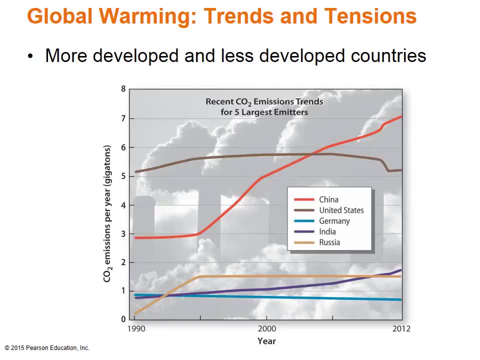 increased their output over the last 15 years as they move towards becoming fully industrialized countries. However, What is alarming is the rate at which China is emitting and has no plans to slow down The Kyoto Protocol agreement signed by many countries in 1997, except for China, India. 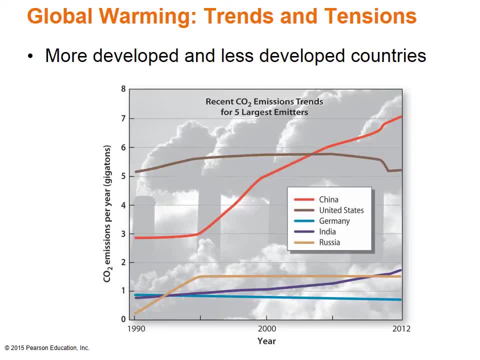 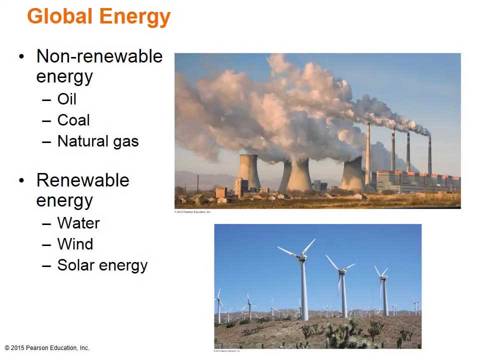 and some other countries would require CO2 emissions to be reduced by certain milestones and dates. Both China and India believe that, even under global pressure to stop, they have the right to continue to develop their economies as they see fit. Global Energy: Energy is a key area studied under Physical Geography and Environment. 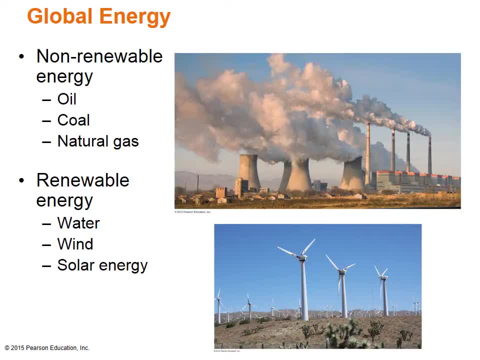 The world runs on energy, which is the capacity to do work. Energy resources are categorized as either nonrenewable or renewable. Nonrenewable resources are natural resources that are considered finite because they are not self-replenishing or they take a very long time to do so, like fossil fuels and 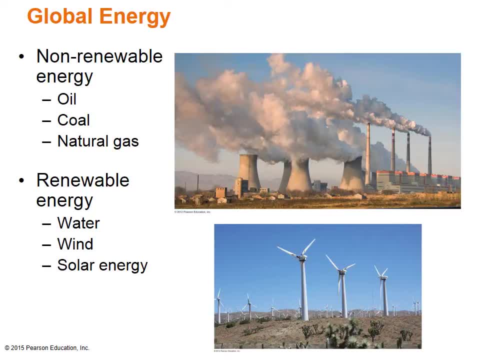 uranium. Fossil fuels are coal oil and natural gas that comes from buried remains of fossil fuels. The fossil fuels are coal oil and natural gas that comes from buried remains of fossil fuels. The fossil fuels are coal oil and natural gas that comes from buried remains of fossil fuels. 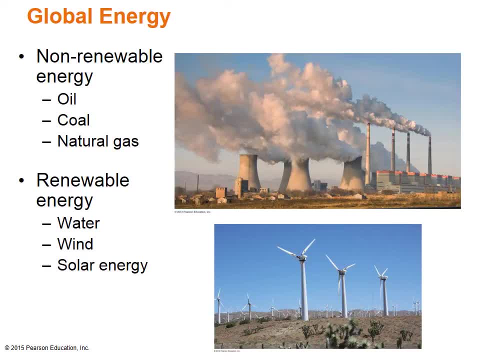 plants and animals that lived millions of years ago. Over time, sand and other sediments covered these deposits, while heat and pressure gradually transformed them. The top photo depicts a coal-burning plant in China. Renewable resources, however, are resources replenished naturally or through human intervention, like planting a tree. Renewable resources include: 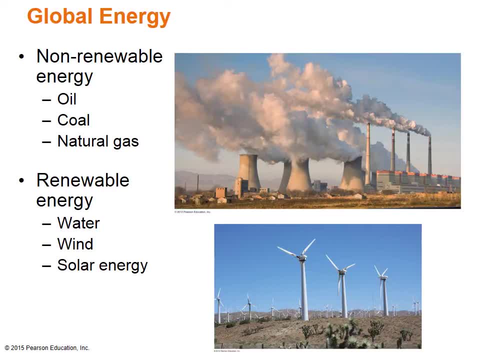 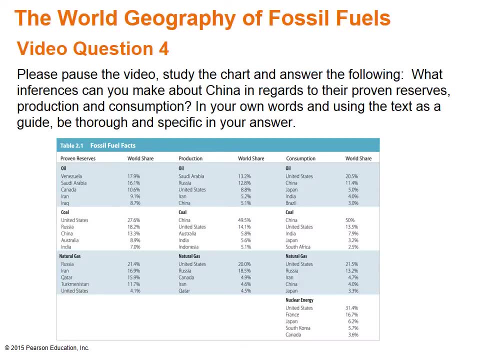 water, wind and the sun. The bottom photo shows a wind farm in California. This chart shows the varied world geography of energy resources, production and consumption. Because a high degree of uncertainty and technological difficulty is involved with fossil fuel mining, the energy industry uses the concept of proven reserves to refer to deposits that are possible. 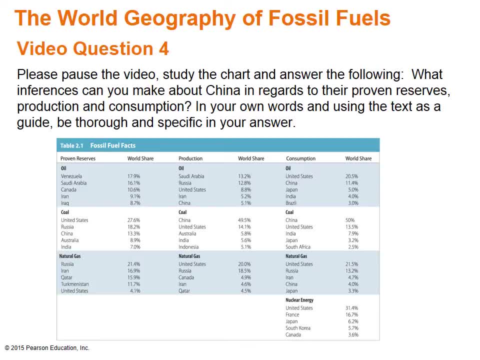 to mine and distribute under current economic and technological standards. End of slide conditions. Please pause the video, study the chart and answer the following question: What inferences can you make about China in regards to their proven reserves, production and consumption? In your own words and using the text as a guide, be thorough and specific in your answer. 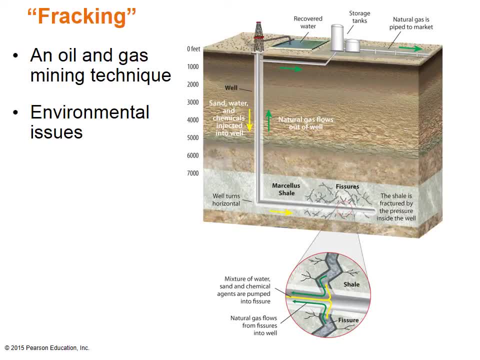 Hydraulic fracking is the latest technology development in the mining of oil and gas. This process forces the oil and gas out of shale rock deep below the earth's surface, as shown in the diagram. If fracking proves unsuccessful, then it would drastically alter the way we produce and trade. 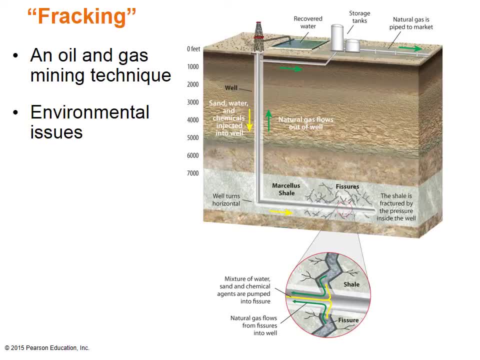 these resources. However, fracking comes with environmental challenges. Fracking requires a huge amount of fresh water, with the possibilities of polluting local groundwater. It also raises the issues of wastewater disposal, local noise and nuisances, And the possibility of causing more earthquakes in the certain geological structures. 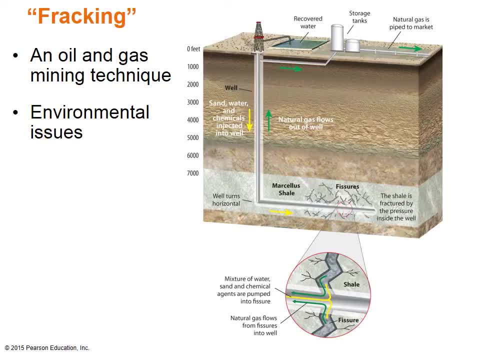 In the United States. fracking is very controversial, but could be one of the greatest solutions to self-satisfying the energy needs in the US if the environmental issues are satisfactorily resolved. This would also be true for China and Russia, since they have a large reserve of shale rock. 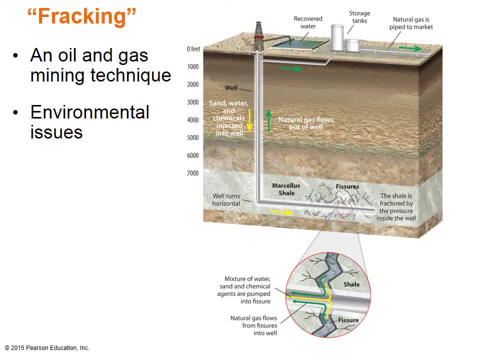 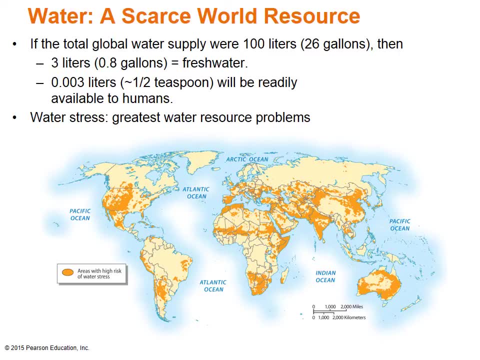 as well. The earth's surface is about 70% water. This means that the surface of the earth is about 70% water. Yet water is the scarcest resource in the world and the most vital to human survival. It is really hard to believe that, out of all the water we see on our planet, 97% of it. 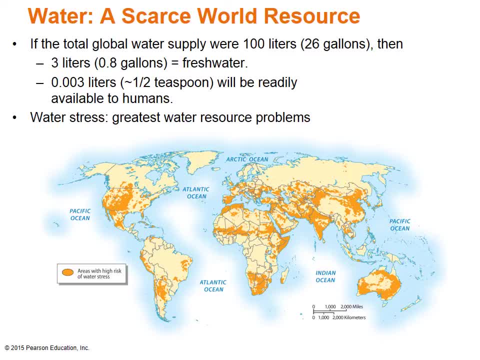 is unusable to humans due the fact that it is salt water And of the 3% of fresh water, 70% is basically unreachable in that it is frozen in the polar ice caps in glacial mountains. In addition, groundwater, which equals almost the remaining amount of fresh water or water. 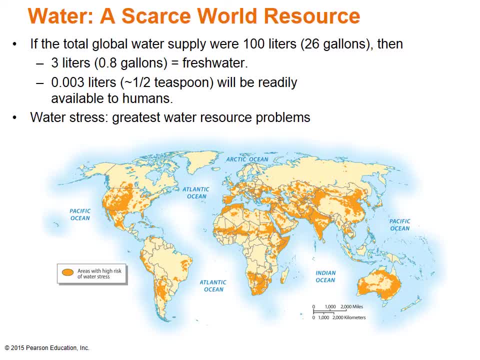 found underground. Therefore, that leaves less than 1% of the world's water in more accessible surface rivers and lakes. In other words, if the total supply of global water is 26 gallons, 0.8 gallons would be fresh water and only approximately a half a teaspoon is readily available to humans. 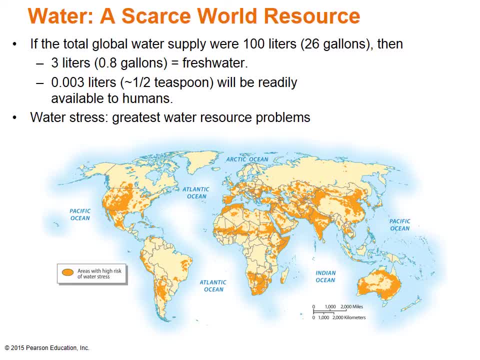 That's not very much, And to combine that amount with it not being evenly distributed across the globe, that makes water stress high on the resource problem list. So what is water stress? Let's look at some examples. 1. Water stress data is calculated by the amount of fresh water available in relation to current 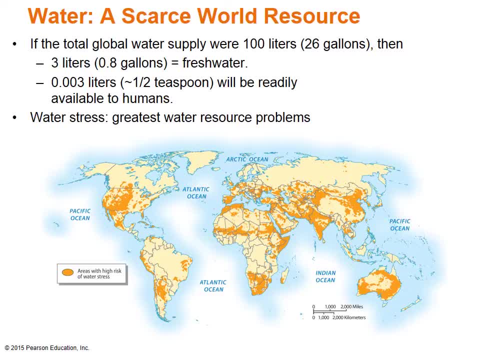 and future population. Water problems also stem from natural global climates that produce wet and dry areas, political controls over river basins and different economies having different water usage patterns. The map shows where water stress is the greatest. Water planners use the concept of water stress for those regions where water is or will. 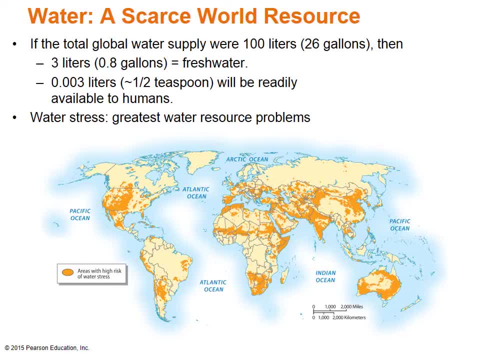 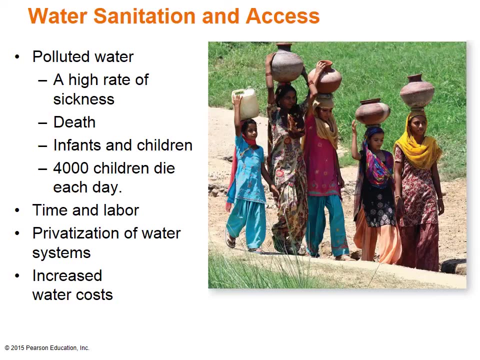 be in short supply because of the combination of high water usage, high water consumption, high water usage, low water supply and the forecast population growth of an area. Unfortunately, people use polluted water when fresh water is not available. This leads to high rates of sickness and even deaths. 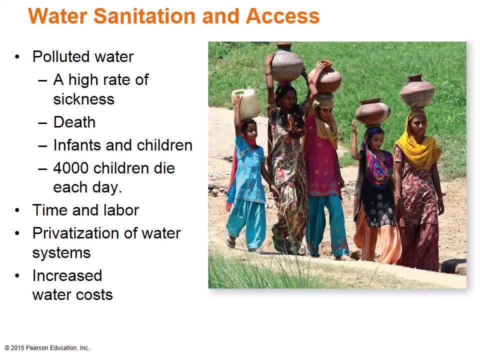 Globally, the rate of illnesses from polluted water is about 50%, according to UN reports, and most of them are infants and children who have not yet built up the tolerance to the contaminated water. It is also reported that almost 4,000 children die from unsafe water and lack of basic sanitation. 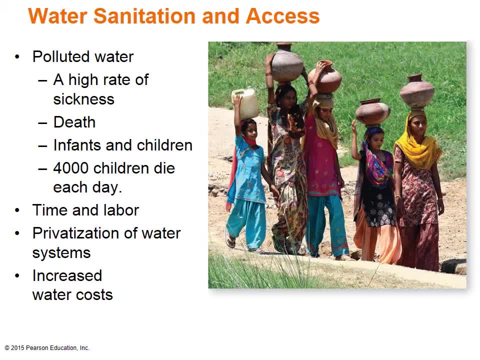 facilities. In many parts of the world, women and young girls spend much of their day providing water for their homes and villages. For young girls, this task often interferes with their schooling. These women and girls are fetching water in the Punjab region of India. 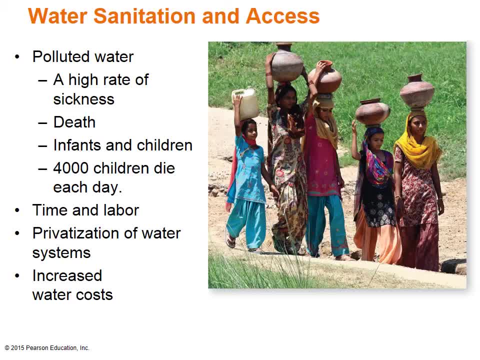 Some recent efforts to help water access have included loans and economic aid to developing countries to encourage the development of private water systems. However, this has proven more problematic to the users due to the privatization of the system. The international engineering firms who upgraded the systems had to recoup their investment. 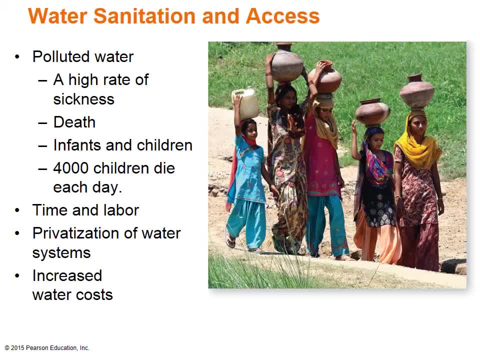 thusly driving the cost up. In Cochabamba, Bolivia, for example, the privatization of the water system in 2000 resulted in a 35% increase in water costs. In response, the people rebelled and rioted With demonstrations that became tragically violent. eventually, the water system was. 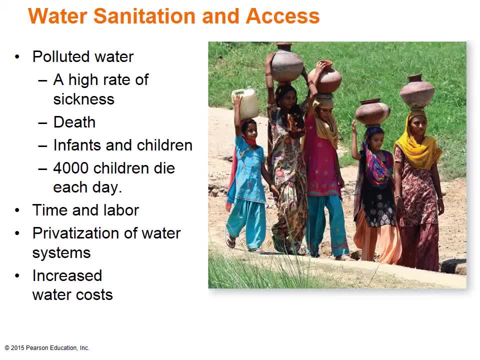 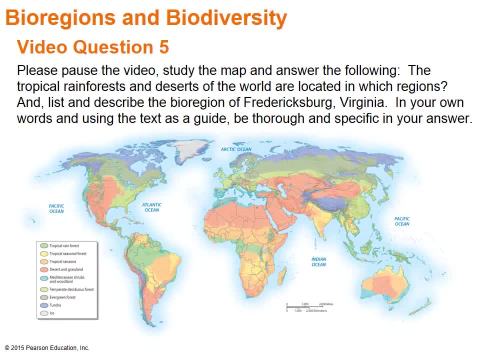 returned to the public control. However, today half the city's population is still without reliable water source. Although global vegetation has been greatly modified by clearing the land for agriculture and settlements and by cutting forests for lumber and paper pulp, there is still a recognizable 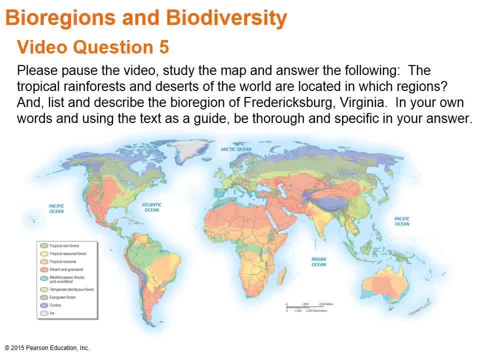 pattern to the world's bioregions, ranging from tropical forests and woodlands to savannas and grasslands, to desert and arctic tundra. Each bioregion has its own array of ecosystems containing plants, animals and insects. 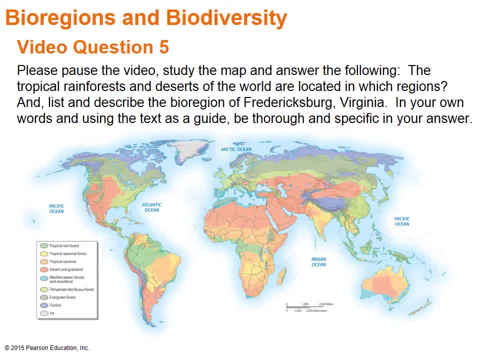 Take a look at Latin America. It has some of the most diverse bioregions in the world. Please pause the video, study the map and answer the following: The tropical rainforests of the world are located in which regions? Also, the deserts of the world are located in which regions as well? 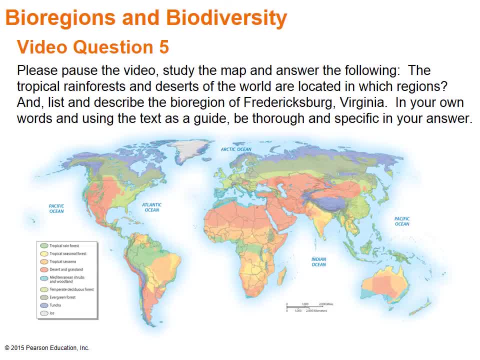 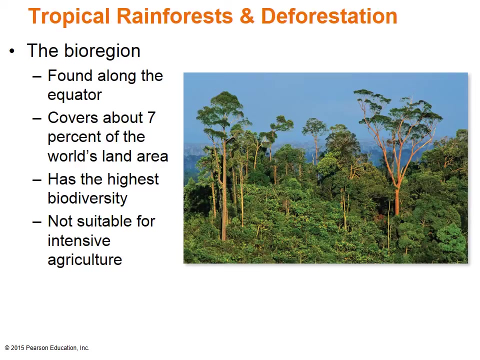 And list and describe the bioregion of Fredericksburg, Virginia, In your own words and using the text as a guide. be thorough and specific in your answer. Let's examine the tropical rainforests in more detail. Tropical rainforests can be found around the equator in the AF climate region. 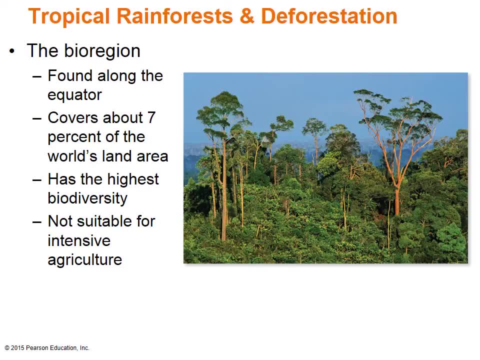 This region has high average annual temperatures, Above zero degrees. There is abundant sunlight and a lot of rainfall occurring throughout the year. With more than 50% of the world's known plant and animal species living in tropical rainforests, that makes the bioregion with the highest biodiversity. 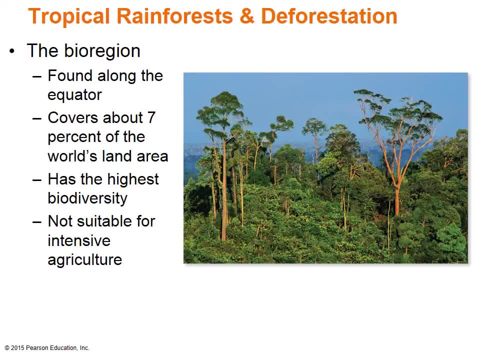 These areas unfortunately are not suitable for agriculture because so little sunlight reaches the forest floors. Since the forests are so thick and dense, most of the sunlight only hits these massive treetops, and most of the nutrients found in the soils are absorbed by the extensive tree. 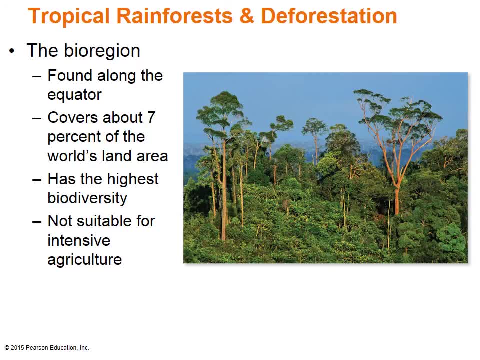 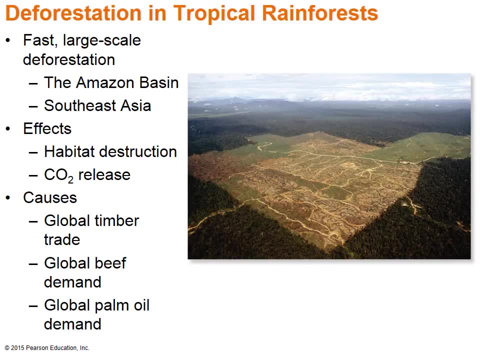 root system. Deforestation has been a huge environmental challenge for our tropical rainforest bioregions. The two hotspots are the Amazonian Basin of South America and the forests of Southeast Asia in countries like Indonesia. Even though we hear more about deforestation in the Amazon, Southeast Asia has been logging. 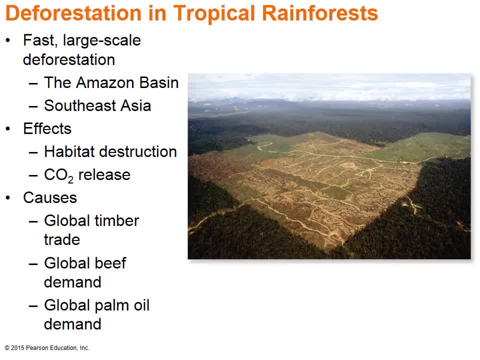 at three times the rate of that in the Amazon. Vital to people and our planet's health and well-being. the Amazon is referred to as the lungs of the world. By the rapid removal of these trees, we are destroying habitats and creating global warming. 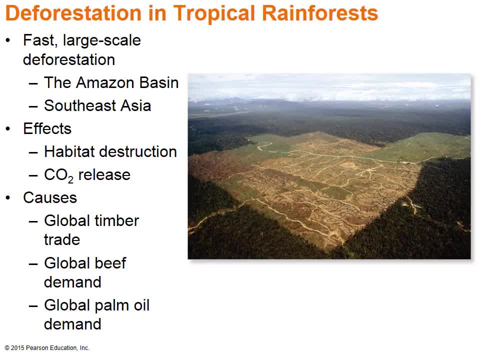 at alarming rates. These trees are used mainly for economic means by the insatiable appetite for wood-based products and beef. More recently, tropical forests have been cleared away to make room for palm oil plantations, whereas the demand for palm oil, a popular cooking oil, has increased. 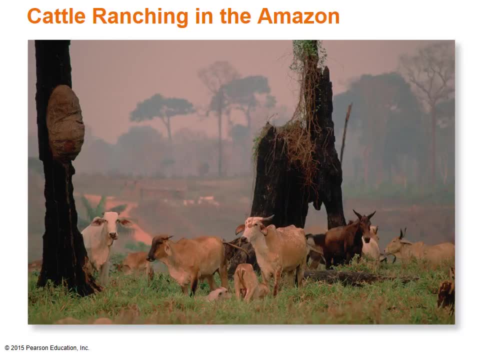 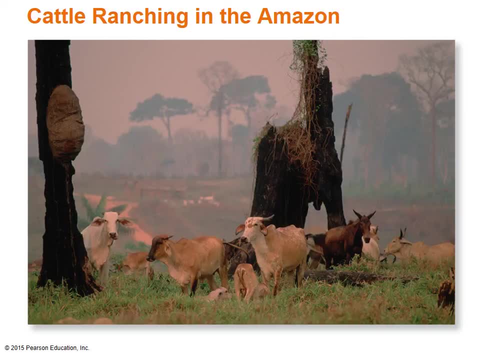 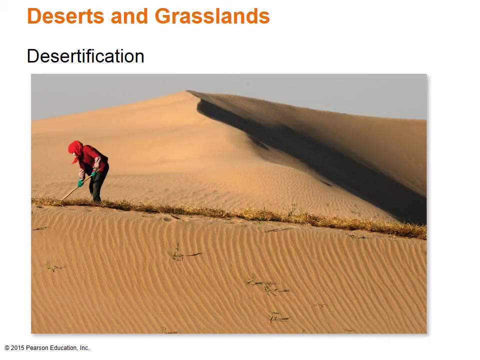 on new pasture created by cutting away and burning rainforest vegetation. Burning the vegetation enriches the soil with nutrients stored in the tree's trunks, but also adds considerable amounts of a greenhouse gases to the atmosphere. Desertification: This is the creation of arid deserts from what was once grasslands. 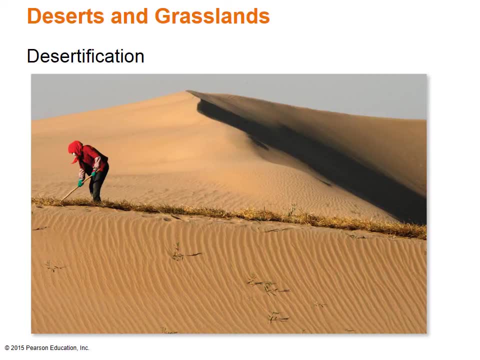 is also another environmental challenge occurring in the world's desert region, Mere Paseo in Cuba. desert regions- Desertification normally occurs when extensive farming is done in the semi-arid grassland areas. In this photo, a worker builds biological barriers using hay to stabilize sand dunes and prevent desertification in the